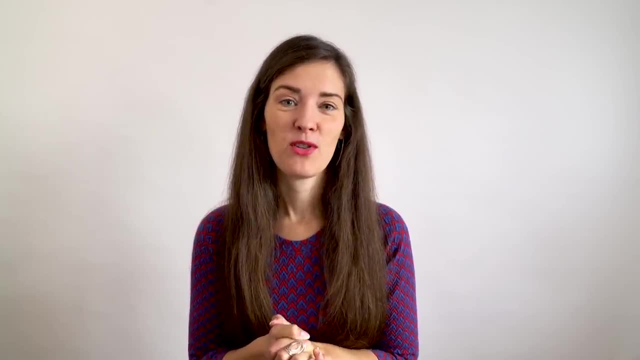 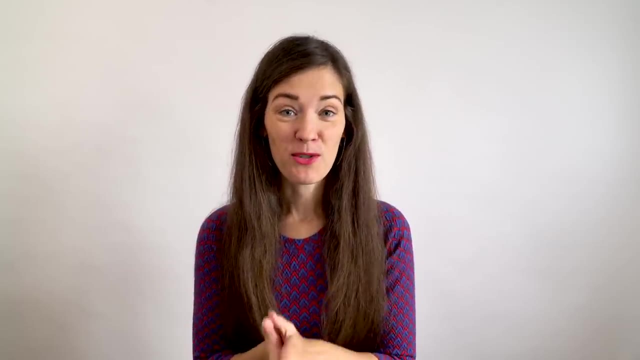 knowledge coming your way. For today's video, I want to show you and really teach you to recognize whether a color is warm or cool. not just the six basic ones, with several tricks. First off, when you choose a garment, a color, it's recommended to match that color to your 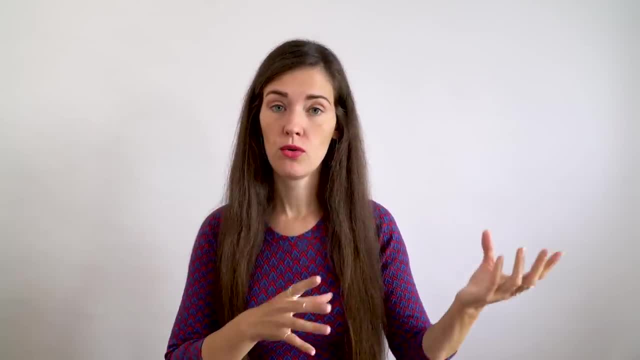 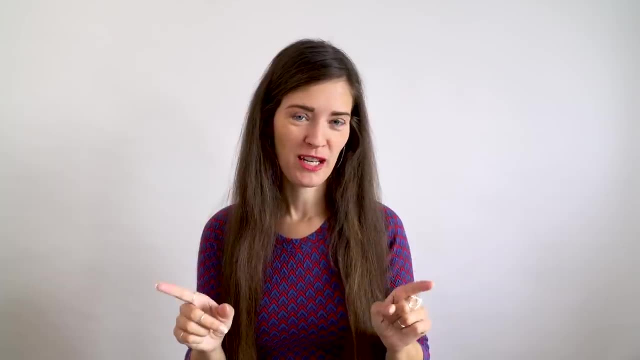 skin undertone. So the rule is: if you are cool toned, you should wear cool colors, and if you are warm toned, you should wear warm colors. If you do not know right now whether you are cool or warm, or maybe neutral, 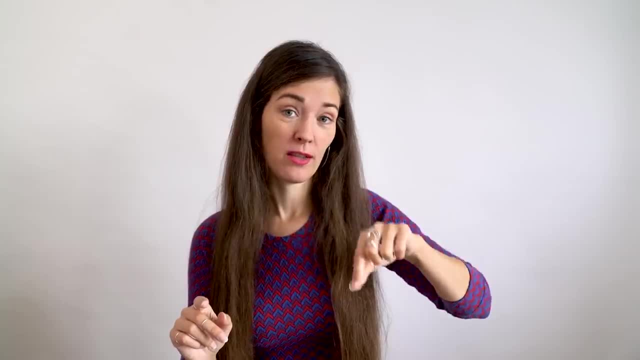 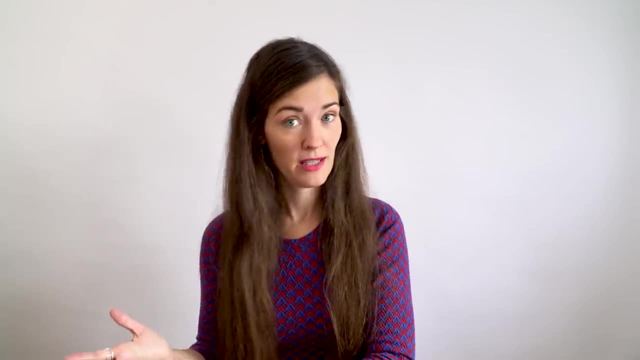 there is a video on my channel, linked here, and also down below in the description, to help you find out very quickly What you are. The problem is when you're in a store and you pick up a garment. it's not always easy to say. 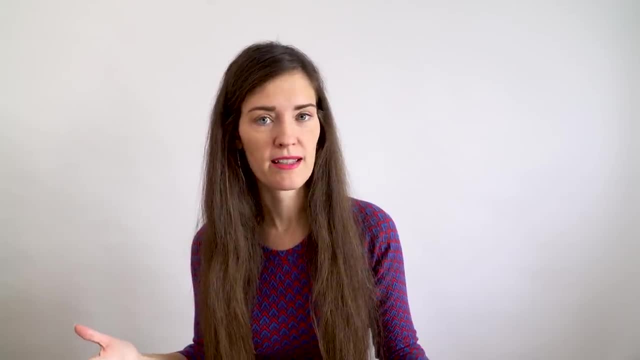 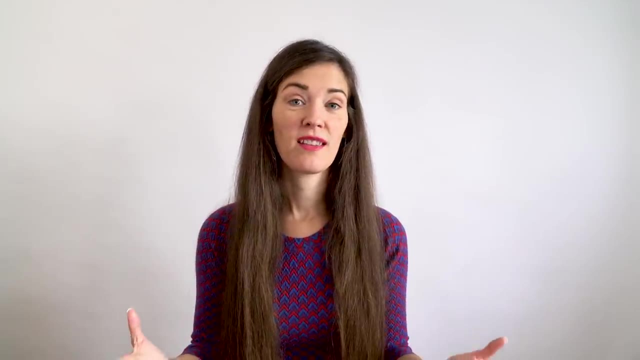 this is warm or this is cool, and the exact color that the garment has. You'll try it on and you might be wondering: does that look flattering? What kind of color is that exactly? The good news is: recognizing cool from warm colors is just a matter of training. 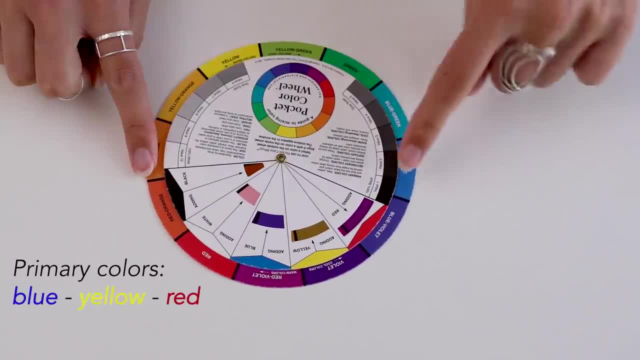 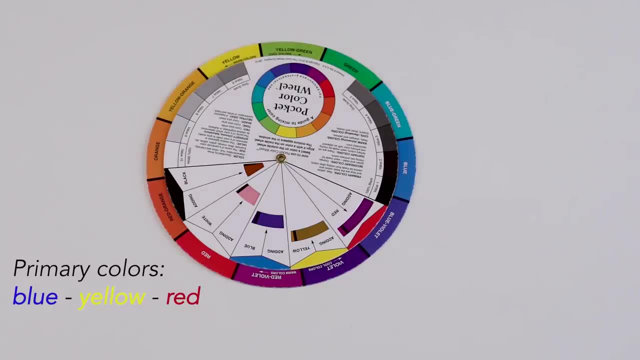 and we're doing this right now. Let's start with the basic color wheel. Blue, yellow and red are the three primary colors which I prefer to call cool hues. Then, if you mix red plus blue, you get purple. Blue plus yellow makes green. 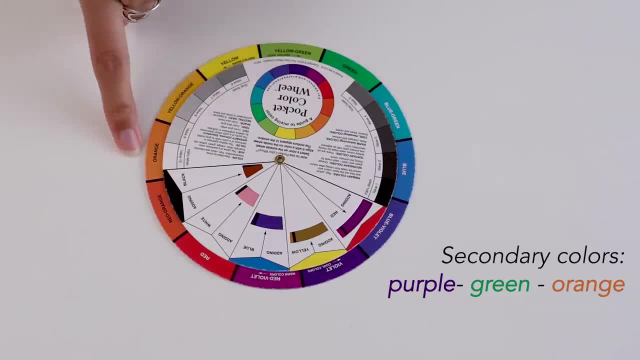 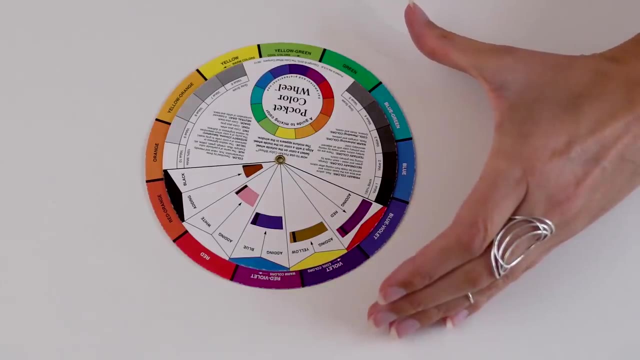 Yellow plus red makes orange. Purple, green and orange are the three complementary colors. Now, from here to here, we have the warm hues Yellow, orange, red And from there to there, the cool hues Purple, blue, green. 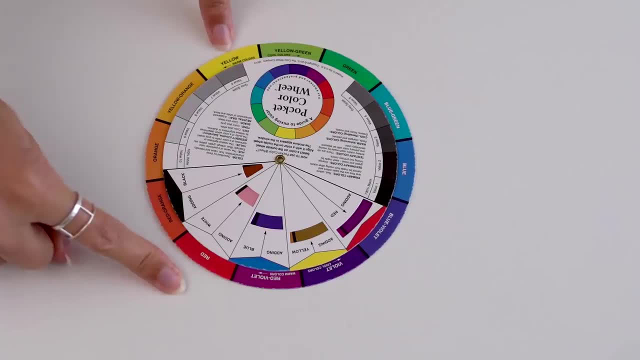 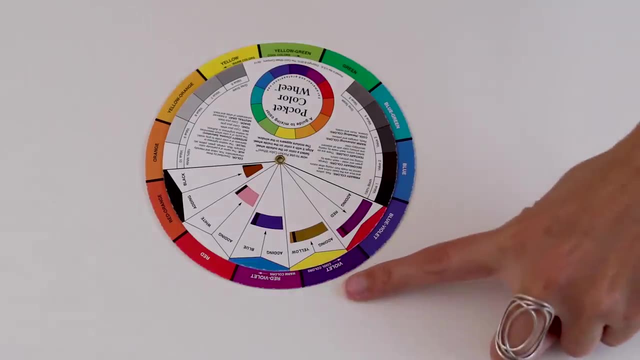 Orange. it's in the middle of the warm range. right It's red mixed with yellow. Both are warm colors. so orange is very clearly warm. But let's take purple. That one's trickier because purple is kind of in between warm and cool. 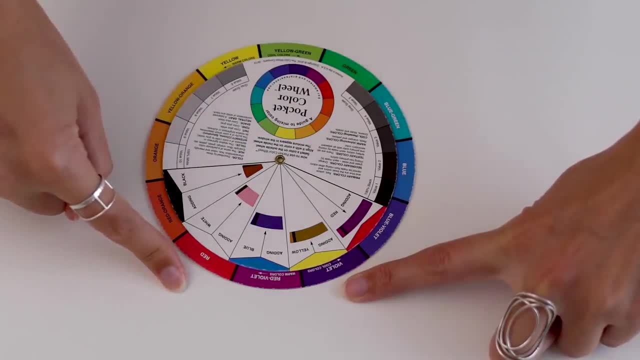 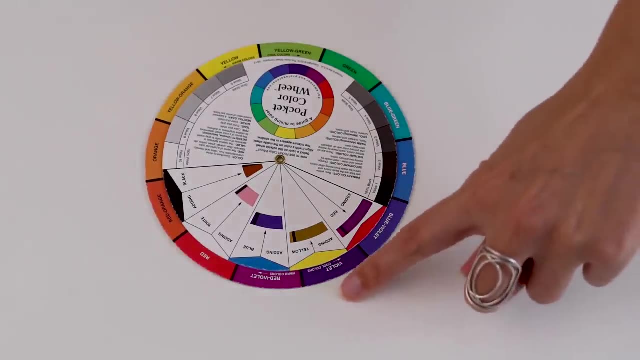 It's a mix of blue, which is cool, and red, which is warm. If I add a bit of red to my purple, my hue turns into red-purple. If I take the same purple and add some blue, it really turns purple. 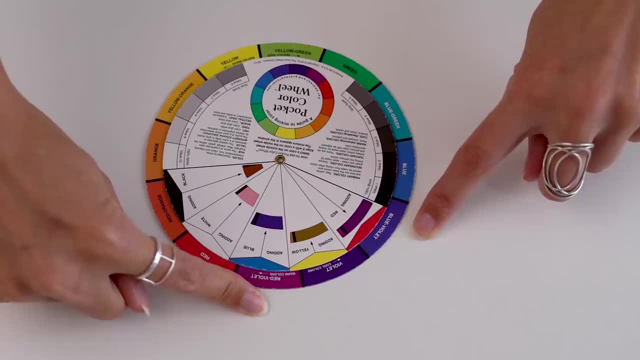 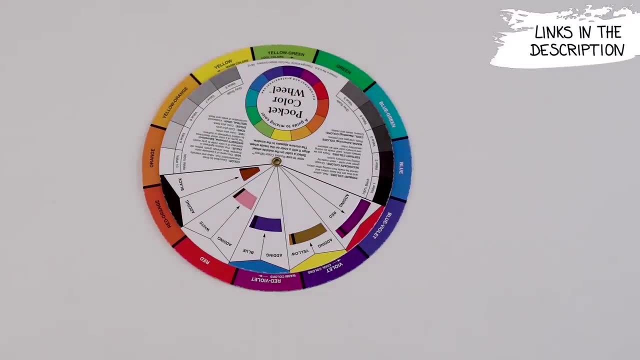 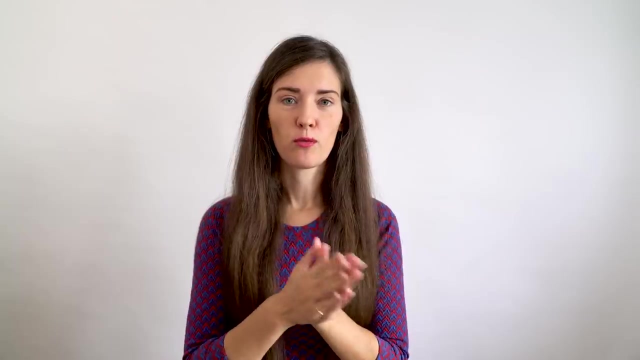 Blue-ish. You can see how the red-purple contains more red and the blue-purple contains more blue. So red-purple is warmer than blue-purple, But all this is purple. So if you ask me, is purple a warm or a cool color? 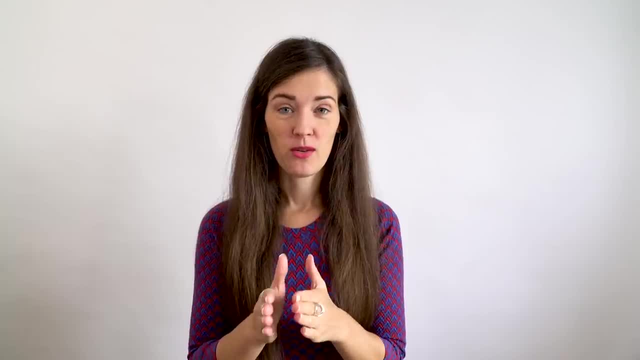 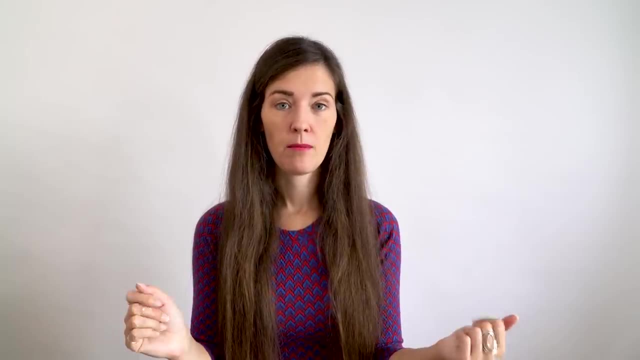 My answer will probably be: it depends. Is the purple that you're looking at containing more red than it contains blue, Or the other way around? That's the actual question. By the way, you hear, celebrity stylists, red carpet stylists. 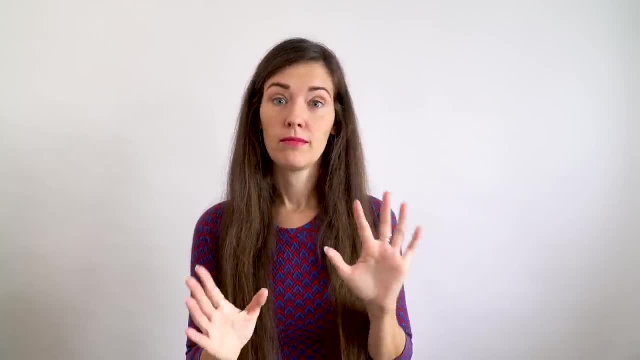 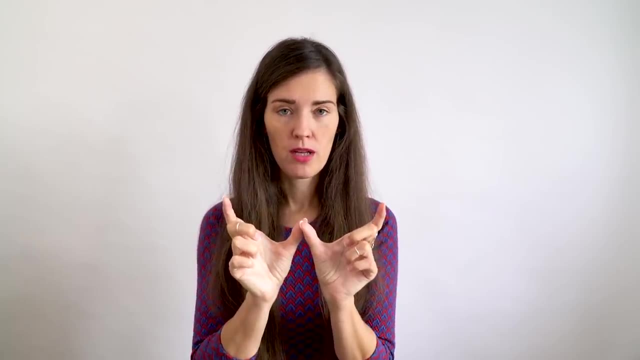 say jewel tones work for everyone. That depends too. I would say Purple, pure purple, really. 50% red, 50% blue. really in the middle is a jewel tone. You could call it neutral because it's in between warm and cold. 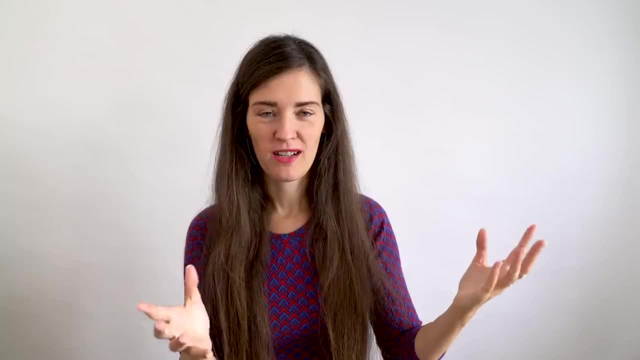 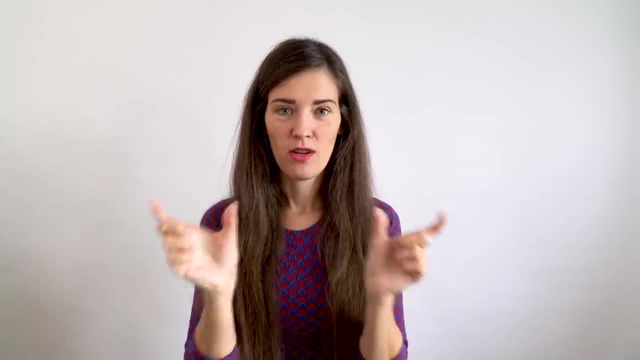 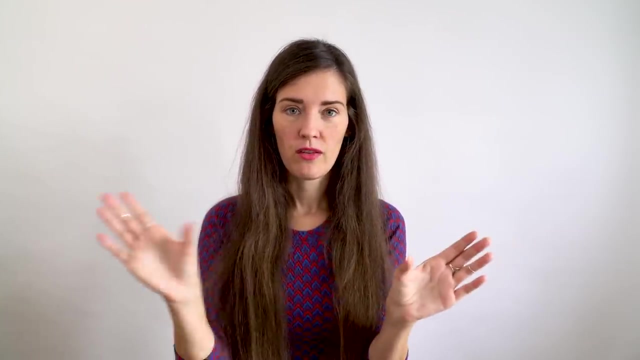 However, the actress you're dressing for that red carpet gala probably is more cool or warm. So, instead of not making any decision and going for the middle ground, work with undertones- that's what I would say at least- and go really towards one or the other. 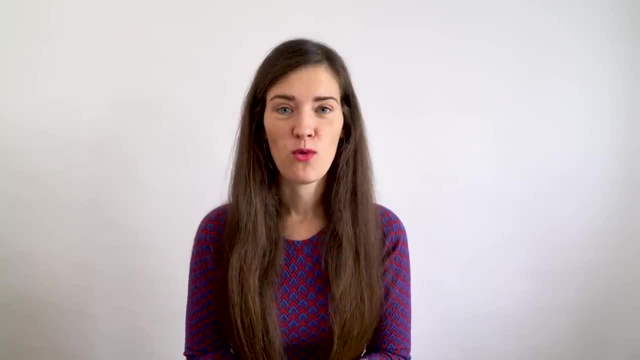 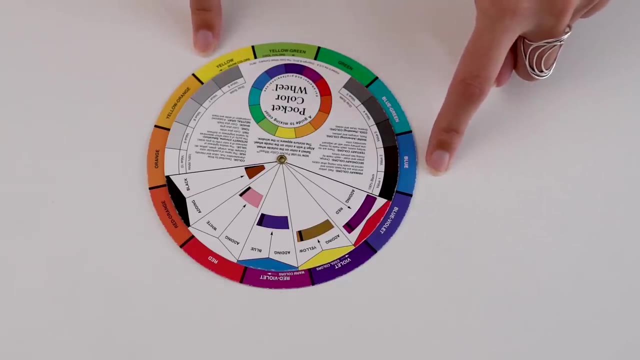 so that the skin of the person will glow and stand out a lot more in the dress. Same thing for green. It's in between yellow, which is warm, and blue, which is cool. So they are warm greens and cool greens. So is the green that you're looking at closer to yellow? 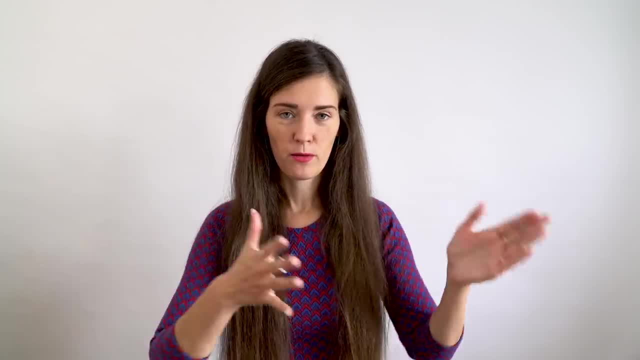 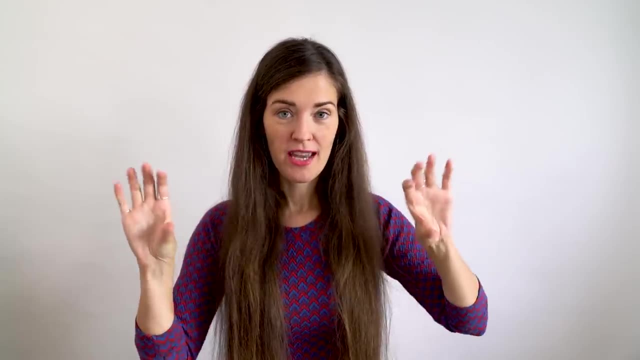 or closer to blue. Okay, so far we have the three primary colors, the three secondary colors. These are the basic six. Apart from purple and green which are kind of on the edge, the other four can be clearly categorized into either warm or cool. most of the time, The problem is when you start mixing hues not in equal proportions to each other, or when you start mixing more than two together. then it gets more complicated to say which color you're actually looking at and therefore whether it's a blue or a green. 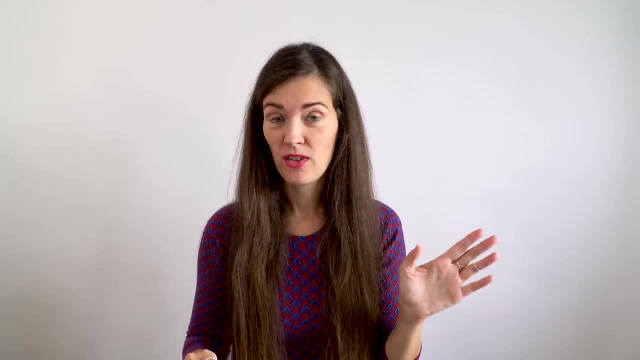 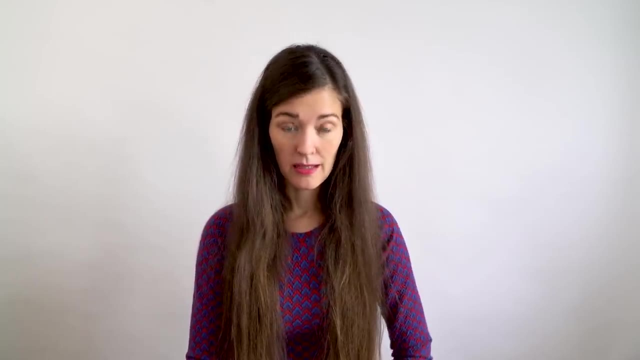 Therefore, whether it's warm or cool, There are also more than six colors in real life, right? So typically, this set has 314.. I'm going to be using this one in a minute, And designers also use bigger ranges than that. 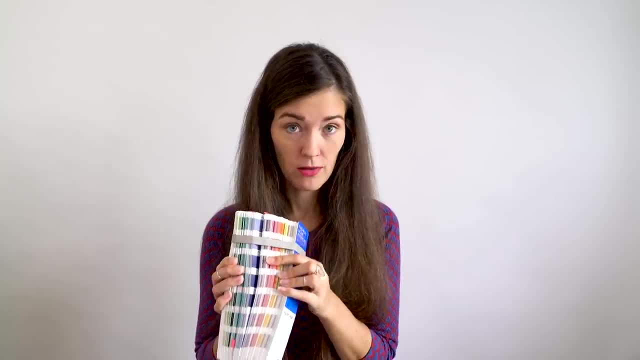 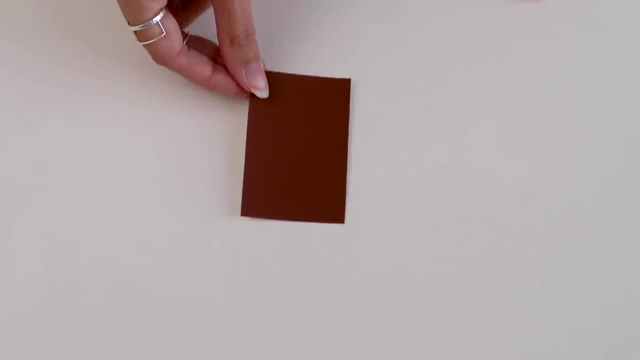 So this is the Pantone color guide for fashion. So, for fabrics, this is the one that I use in my job. It has many, many more options. Let's take this dark brown as an example. Is this warm or cool? If it's cool, then it should contain more blue. 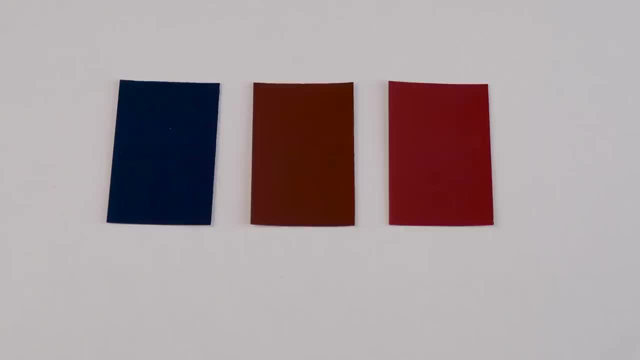 If it's warm, then it should have more red in it. That's why I'm putting a red and a blue next to it. Seeing the three like this, you can tell that the brown is closer to the red than to the blue. 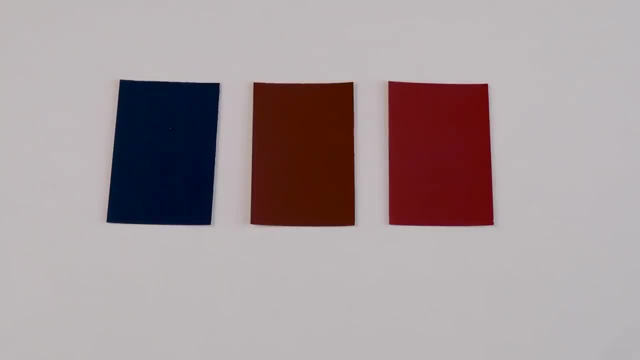 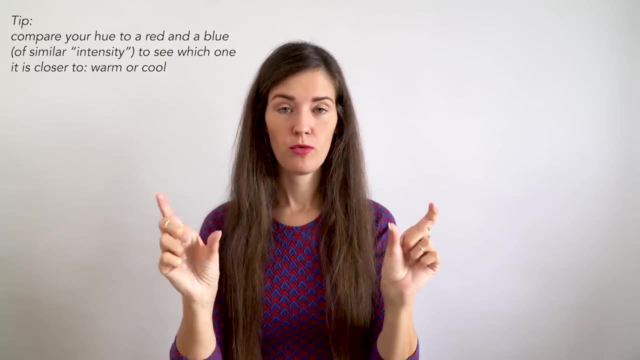 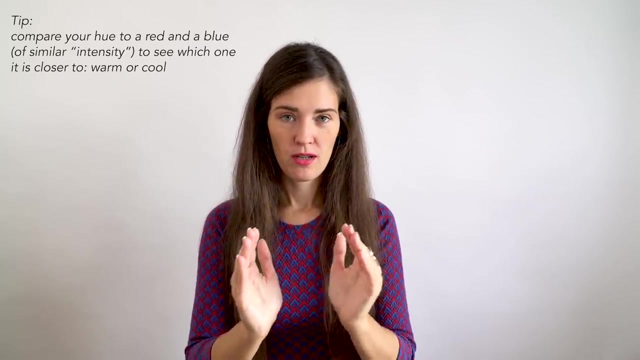 So this brown belongs in the warm spectrum. Brown could be either cool or warm, but this one is warm. Conclusion: When you put your hue in between a red and a blue of similar intensities, I would say it always makes it a lot easier to see whether your hue goes towards warm or towards cool. 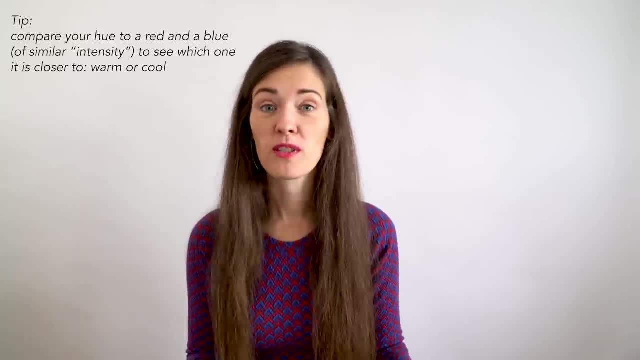 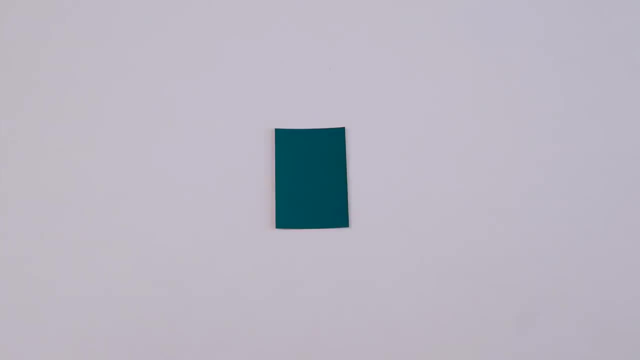 It's a very easy trick if you don't know where to start, and it works most of the time. Another example: this is a blue-green, So in theory it's a cool hue, which it is. Blue and green are hard to differentiate for the human eye and also culturally. 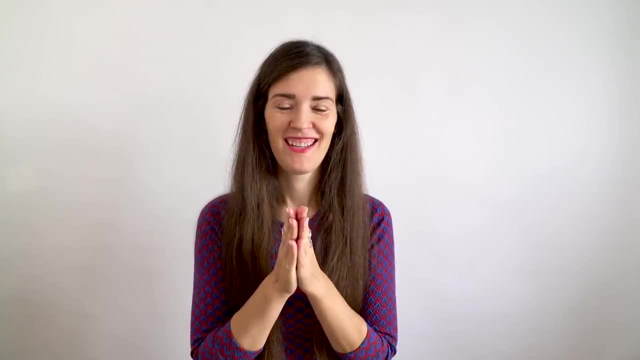 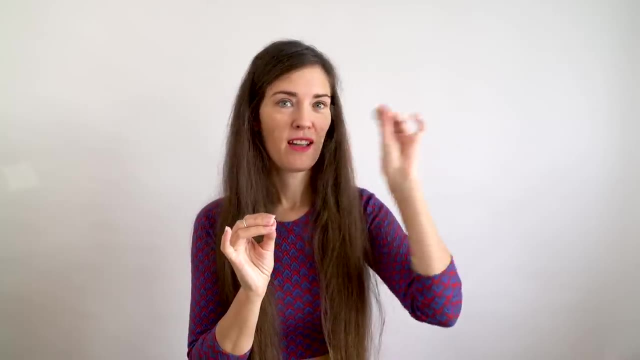 There are languages where blue and green are the same word, For instance, in Vietnamese. correctly it's blue. If I'm wrong, I think you say the same word and then you have to specify: is that the blue of the sky or the blue of tree leaves? 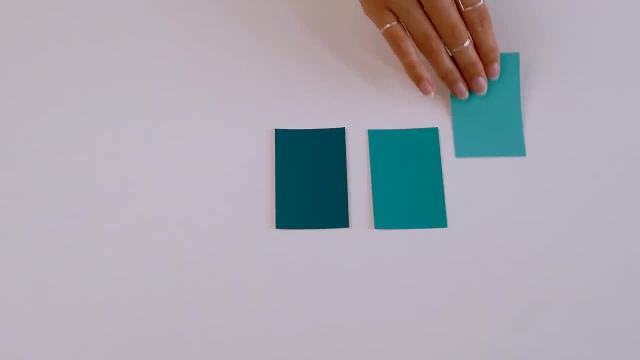 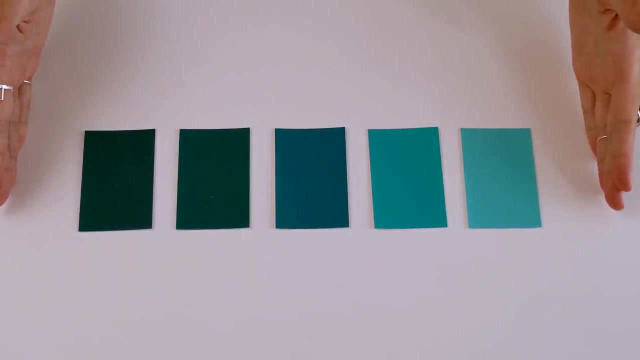 What happens? if you add white to that hue? You get a sort of aqua-green color. And if you add black to the hue progressively, like this, it becomes a sort of dark blue with a touch of green. These five cards have the exact same hue. 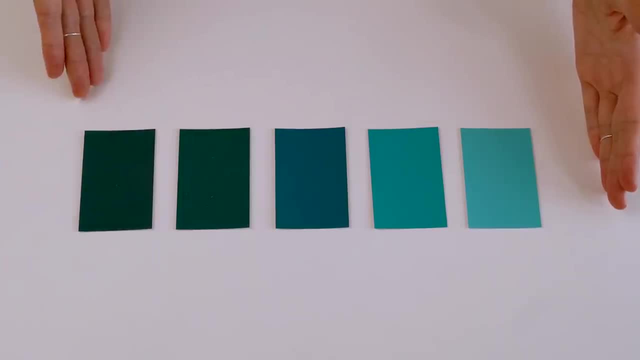 That's why I call them hue and not color. These are five different colors, but it's one hue and therefore the same temperature. They're all cool. The only difference is that in one direction I'm adding white and in the other one I'm adding black. 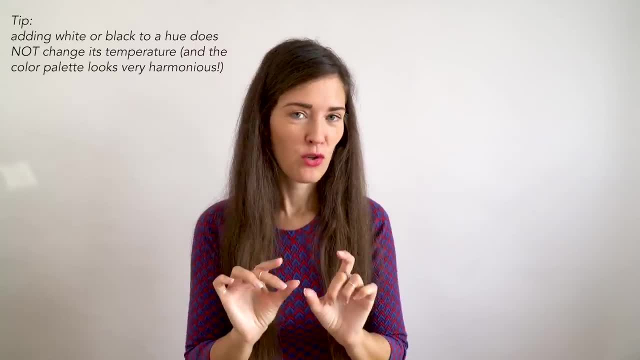 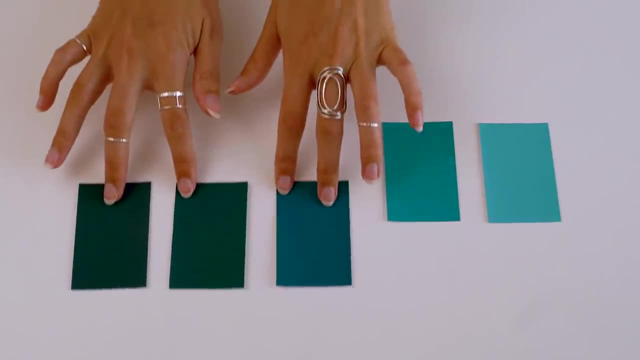 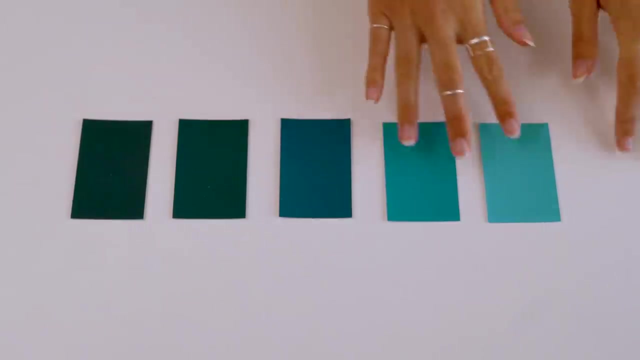 adding white or black to a hue does not change its temperature. Also, if you combine these three or these three in an outfit, you will have the perfect harmony. It's really easy to look at. It's the same family. It's easy on the eye. 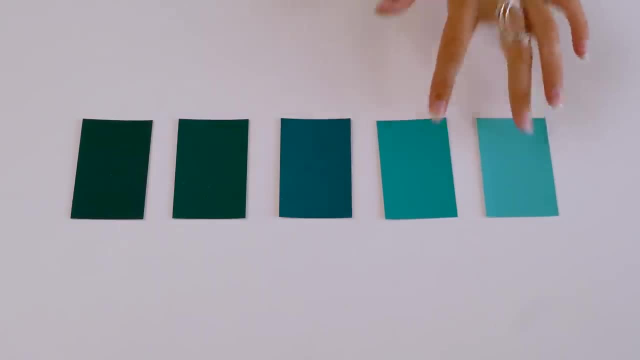 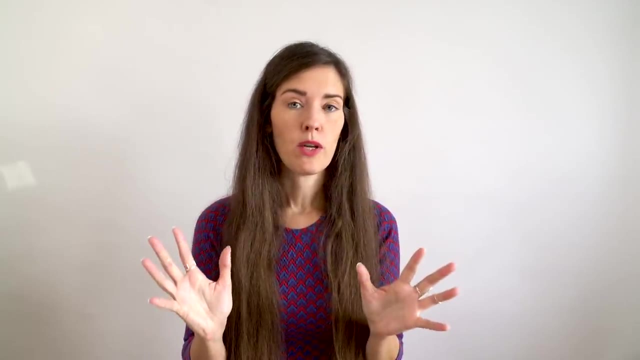 You could also pick. You could pair these with white or the darker ones with black, Also very easy. If you're looking for color palettes that look harmonious, this is absolutely the way to go. You will hear people tell you things like: 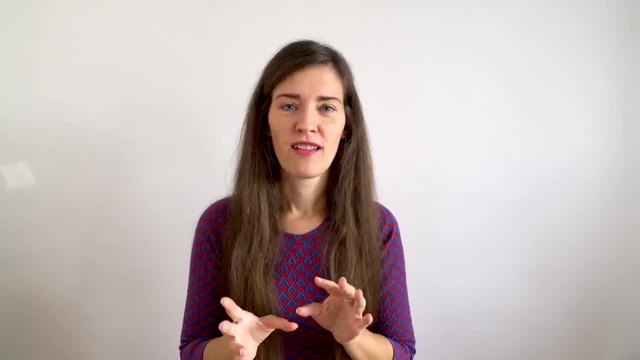 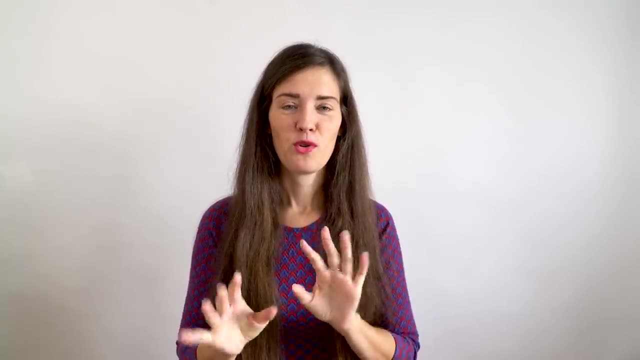 oh, you look so well put together and your outfit looks so cohesive, no matter what you're wearing. It's only about the colors, But I'll go into more details about building a color palette for your wardrobe in the next episodes of this series. 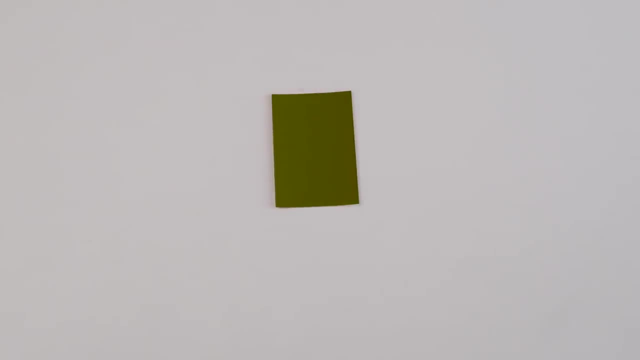 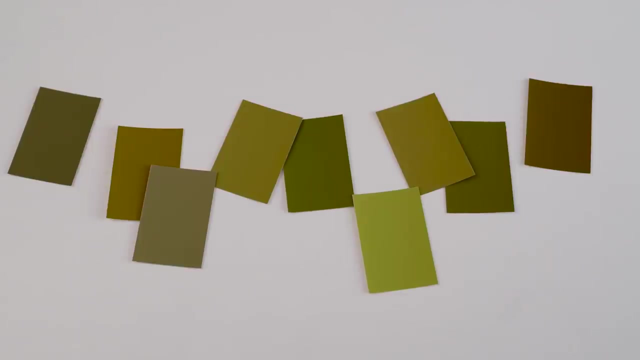 What about khaki? There are many different khakis. This is khaki, these two, this one too. If you saw any of these individually, you'd probably all call them khaki, because they all contain some yellow, They all feel warm. 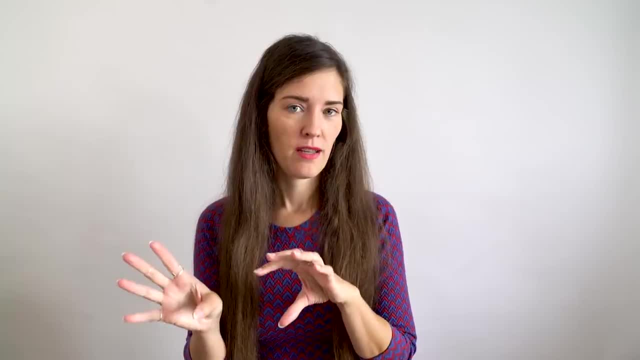 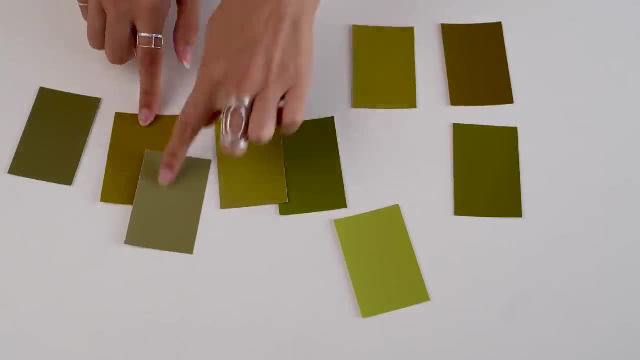 They all are technically warm, Yet I can still group them and organize them in a way as to see which ones are warmer than the others. I have three that are more yellow. The others contain more green, AKA some blue in it, so they're cooler. 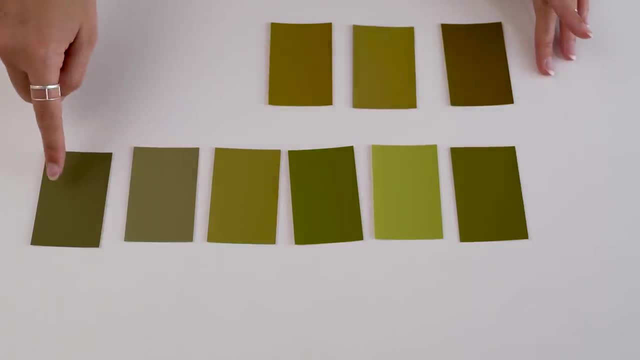 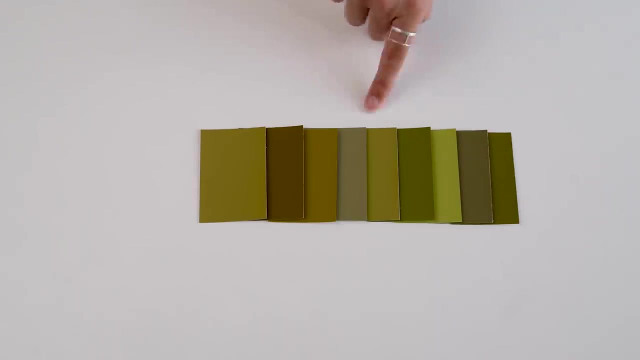 If your undertone is very warm, these three khakis that are more yellow will look even more flattering on you than the others. It gets more obvious if I overlap the cards in one single row: This side is more yellow and that side is more green, AKA cooler. 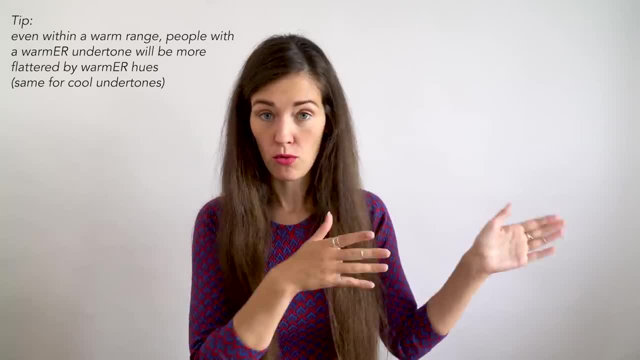 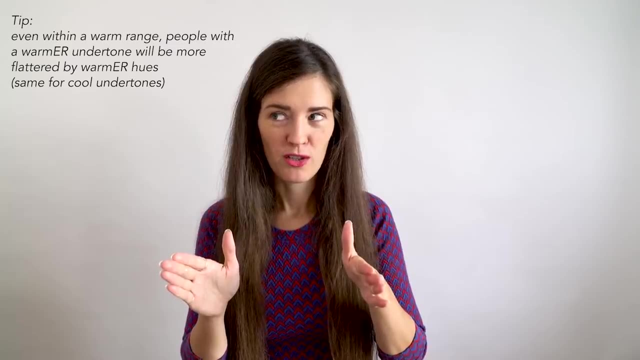 Conclusion: Even within the warm spectrum or the cool one, you can still play with temperature. If you're very warm toned, you can go for hues, colors that are very warm, and you will have an even better effect on how much you glow in your outfit. 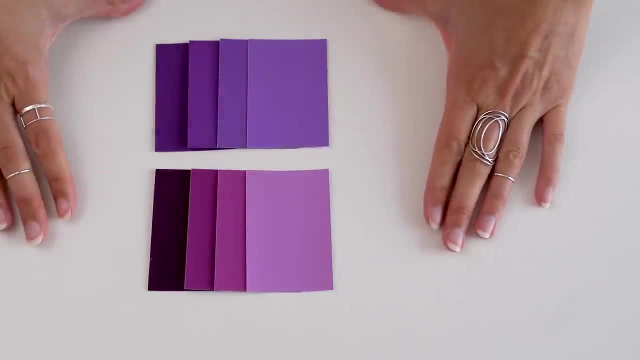 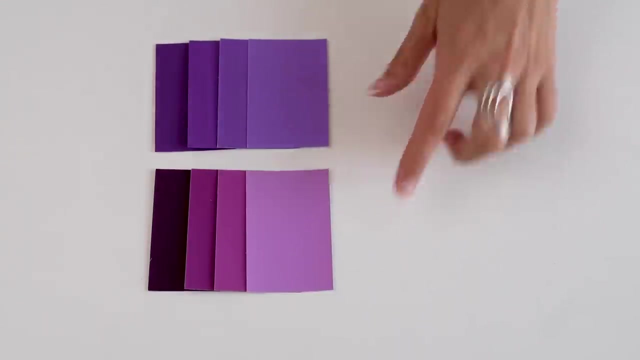 I want to show you another example with purple. See these two sets. they're both purple. Everything here is purple. However, this row contains more red. Can you tell? The darker ones are not so easy to recognize and the light ones are also not so easy. 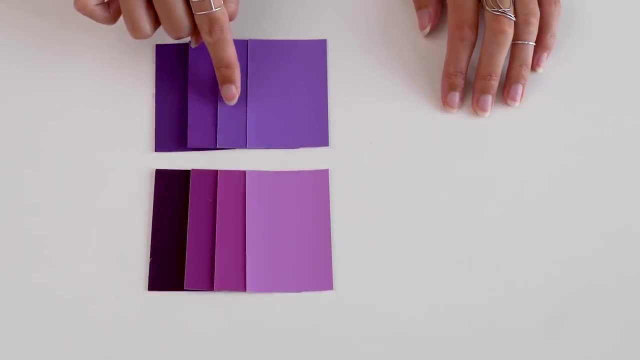 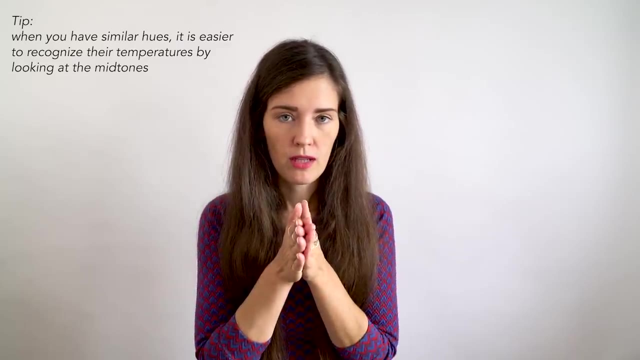 But somewhere in the middle you will see the difference between this and this card Conclusion, Where you're looking at hues that all seem similar at first sight. look at the mid-tones and it's easier to recognize the temperature. That's it for today. 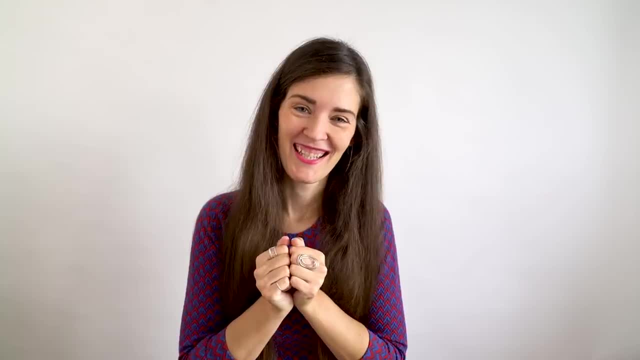 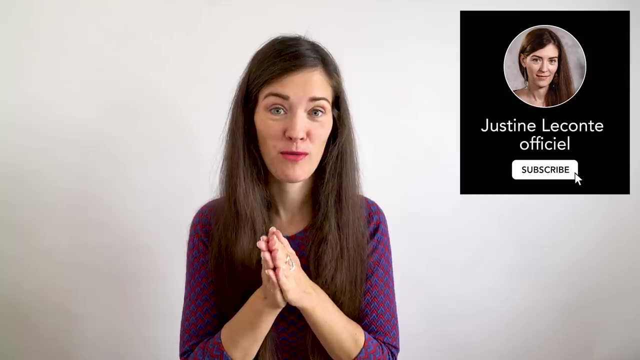 Thumbs up if you enjoyed this little demo. Thank you so much. In the next episodes I will show you how to create color palettes for warm versus cool undertones. If you're interested, subscribe to my channel before you go. watch the next video. 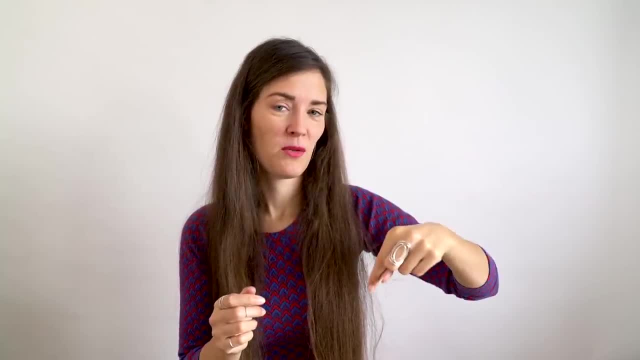 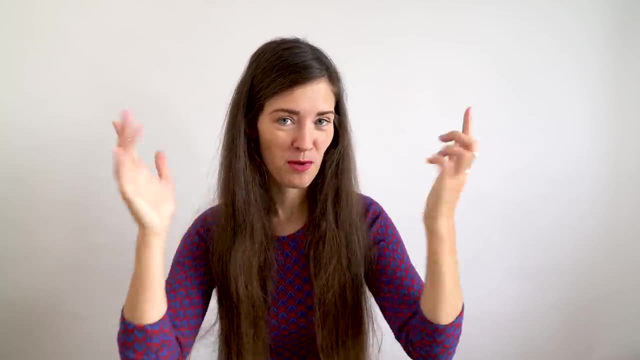 In the meantime, this one, also linked down below, is a video about what the colors you wear say about you, The message, The message that you're sending to other people's eyes, So you can start thinking about which colors you enjoy wearing.